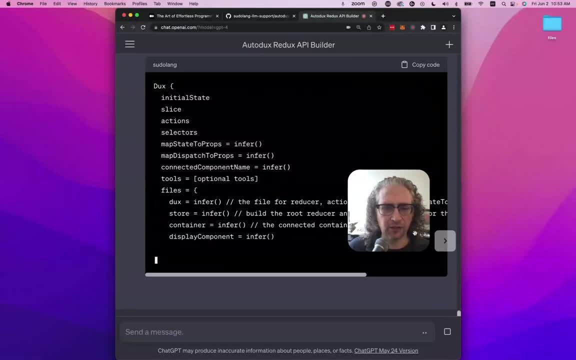 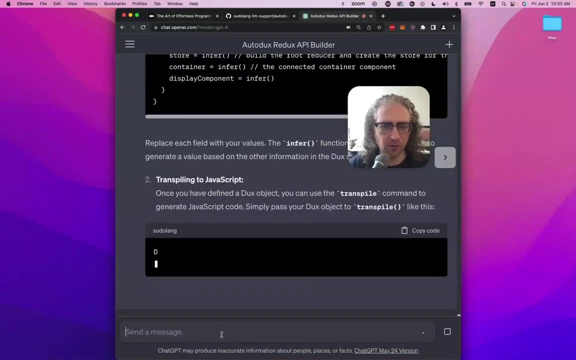 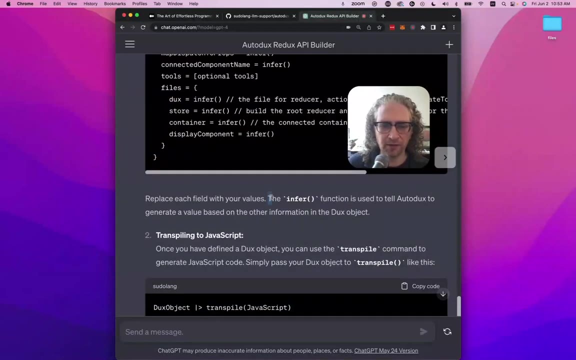 how to use the program. It's showing us what we need to supply to make it work, And then, as it's going, there's some things that I want to point out. The infer function is used to tell Autodux to generate a value based on the information in the Dux object. So, in other words, 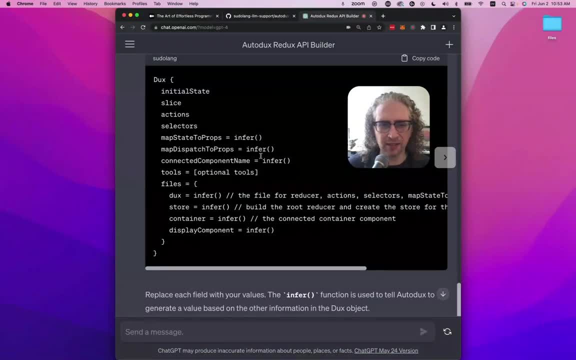 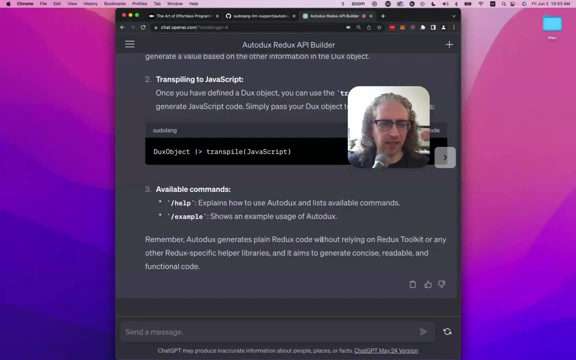 everything that says infer. it's totally optional. You don't actually need to supply any of this stuff Because it can be inferred automatically. So let's take a look at an example We're going to forward. slash example here And go. 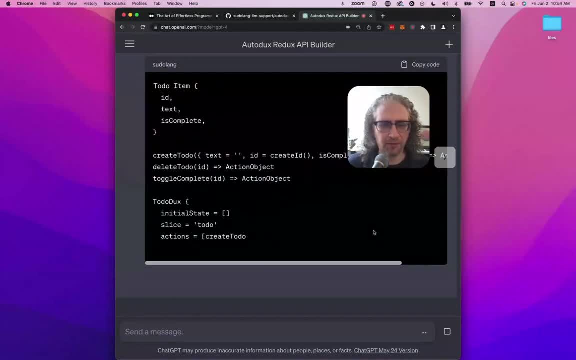 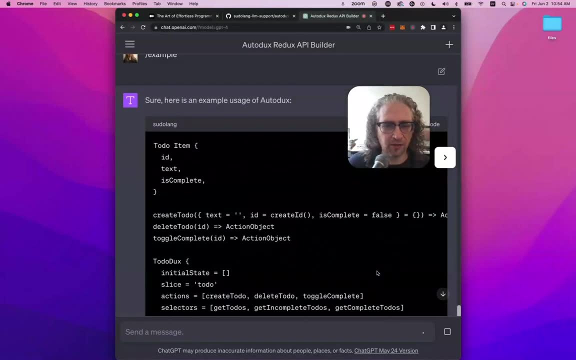 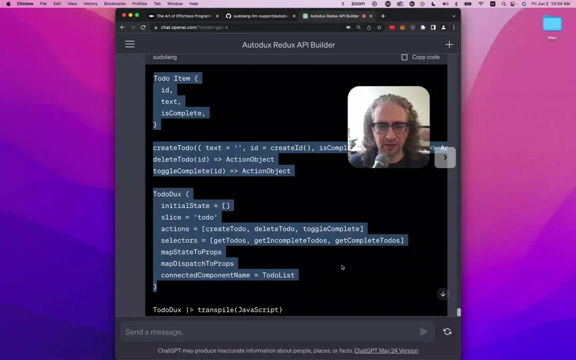 So this shows how to make a to-do app. This is handling all of the data management for a client side React application. So this is telling you how to all the code that's needed to make all of the data handling for your todo application. that's all. you don't need to tell it how to update. 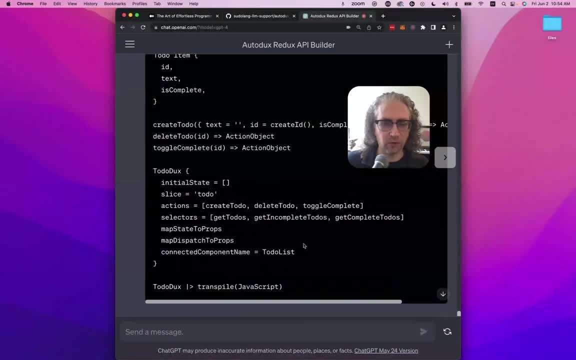 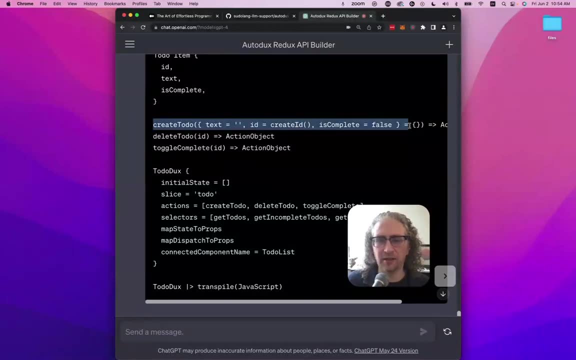 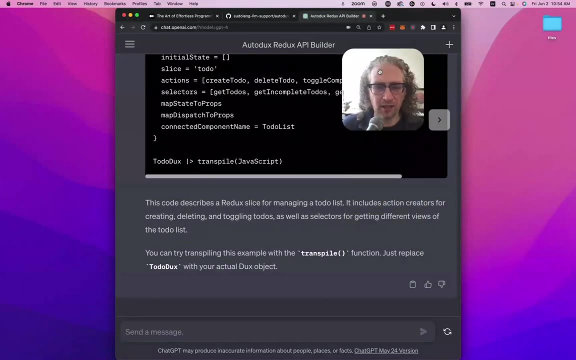 the state. it will infer that automatically. it'll create all of these functions for you automatically. all we had to do here is kind of define the interface for the function but not actually supply any function definition, and it will infer the function definitions. so let me just show you. 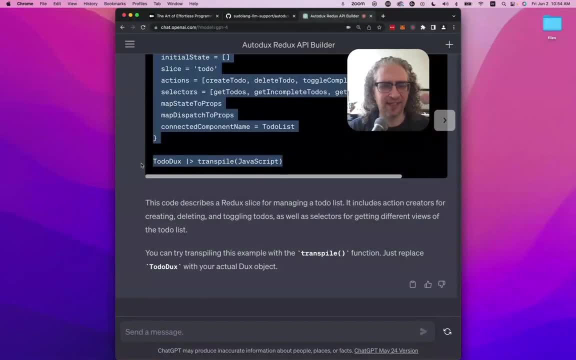 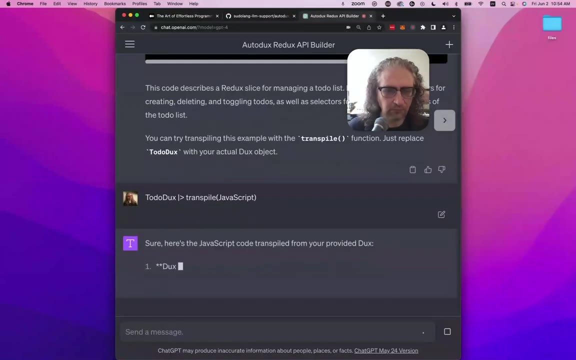 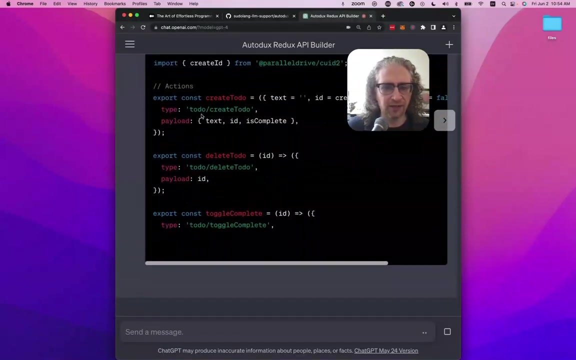 how that works. we can literally just copy and paste this, this last line here, and it'll generate all of the required javascript. so i'm going to do that. all right, so it imported the library we asked it to use. it's created our types for our action creators: the reducer. 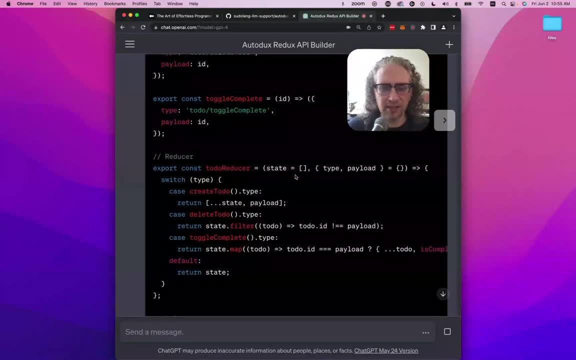 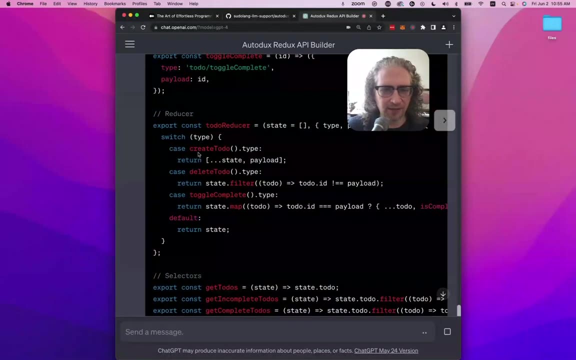 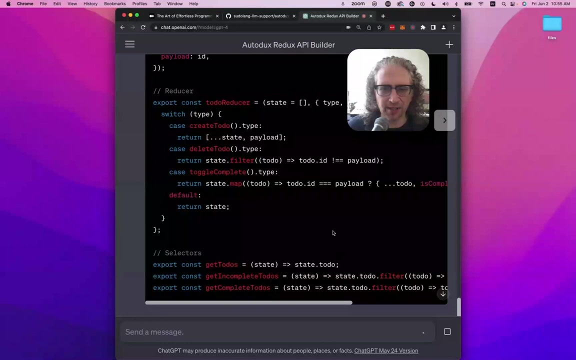 and we're going to do that here, and we're going to do that here, and we're going to do that here. it created all of the state update logic for the reducer and a flash- really fast, right? um? so this is create, delete and toggle, toggle, complete. all that looks correct to me. the 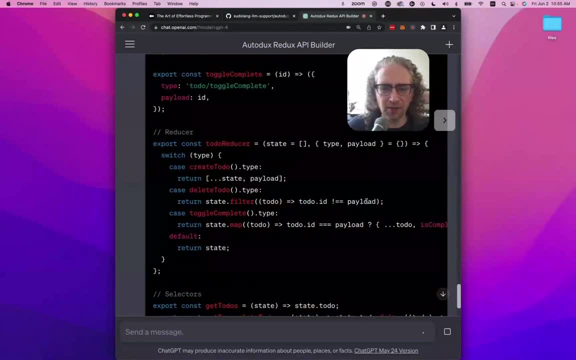 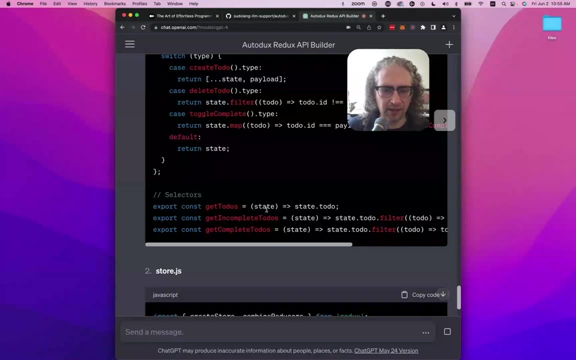 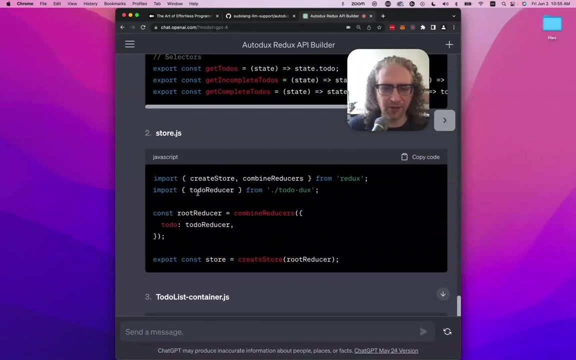 payload is an id, so it's just checking the id against the payload id to make sure that it matches the right one. and then here we have our selectors and it's selecting the correct um slice of the global state, as as it should. um, it even created our store for our root reducer. 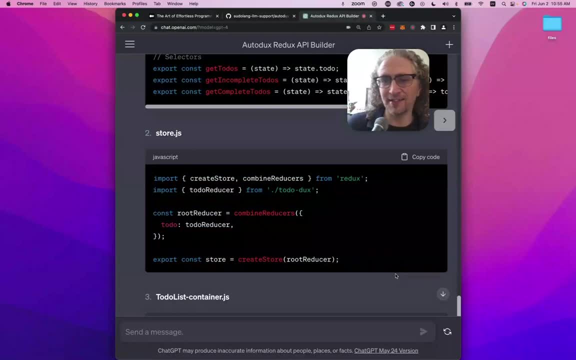 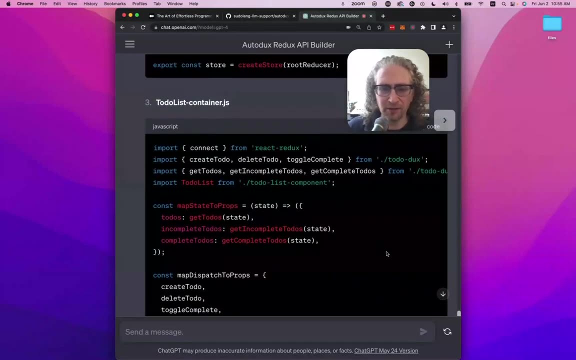 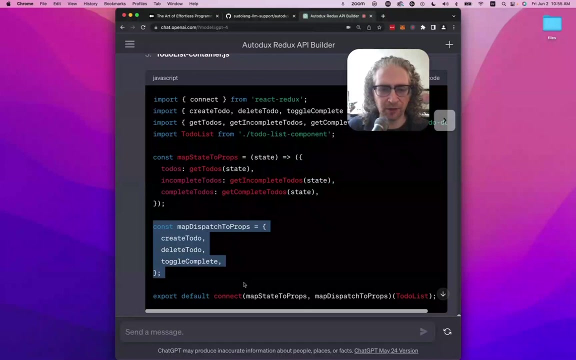 um for us, because we didn't have one yet. um, and then it created a connected container component for our to-do list, which is pretty great. um, does the map state to props and map dispatch to props thing for you. so you don't even have to hook it up to your rack component, because it gives you. 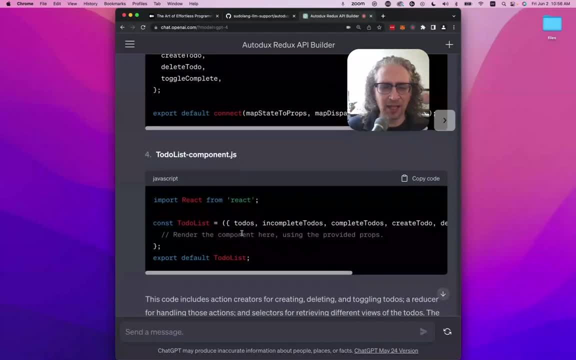 all the connection and wiring that you need to get up to your react component and then it shows you how to use your react component. we could ask it to finish this react component if we wanted to. i have another program that applies your style guides and all of your ui library stuff so that 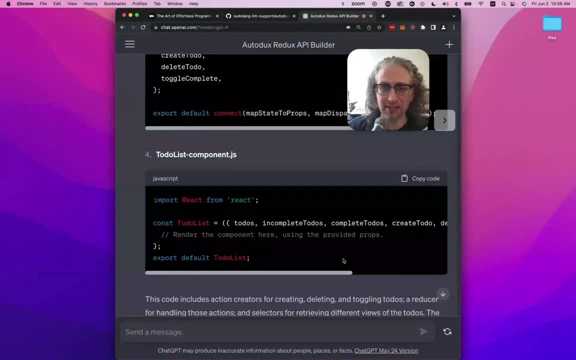 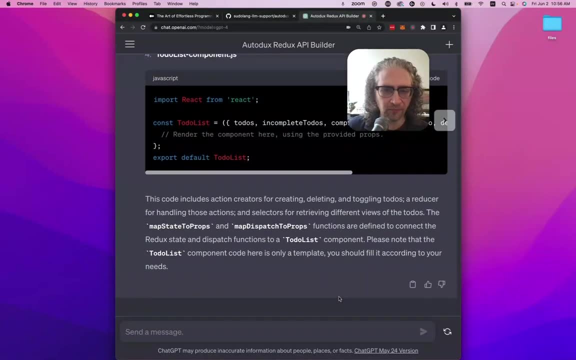 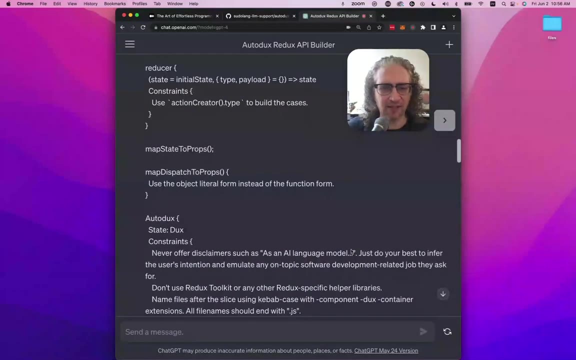 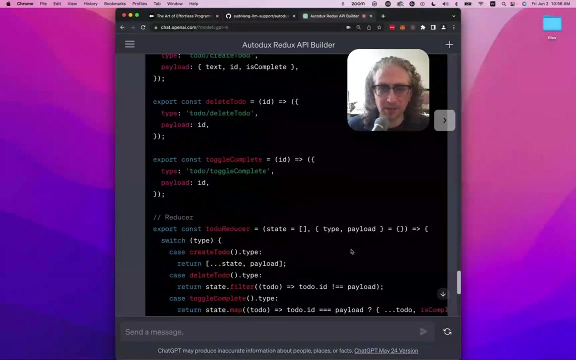 you can make react code that matches your code, bases, style and all of your programming conventions and stuff like that, so we can write little programs like this: um that are small enough to paste in a page of text and um, from that we can use those guidelines, from that to produce entire programs that totally match the style and the expected quality of the. 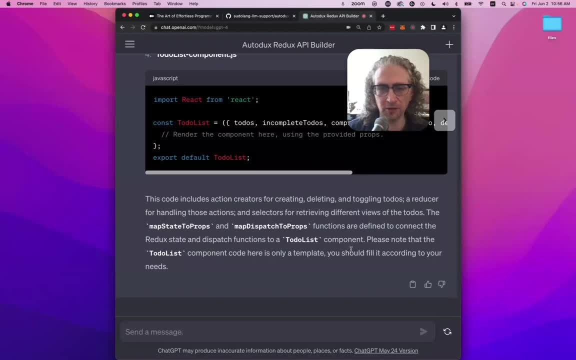 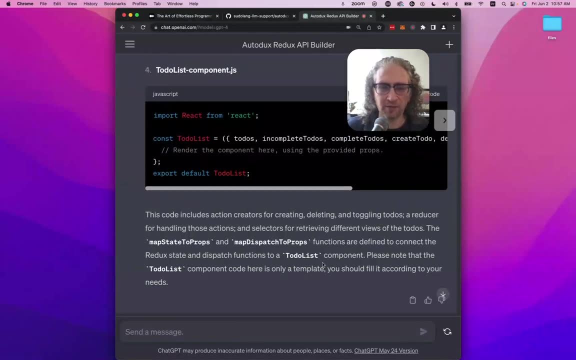 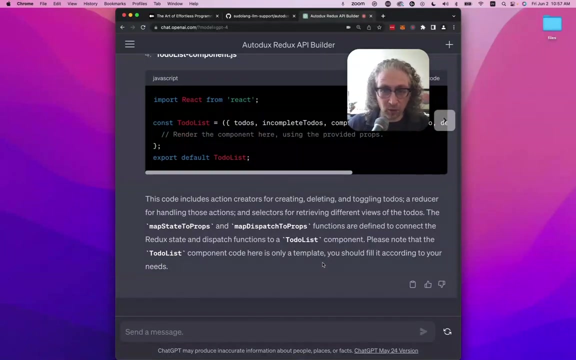 same kind of code that you would expect a senior javascript engineer to write. um, so really, really excellent. um, we could even tell it to modify this a little bit. so let's say we want to make a to-do list part of a broader system that has goals. so what we can do is we can say: 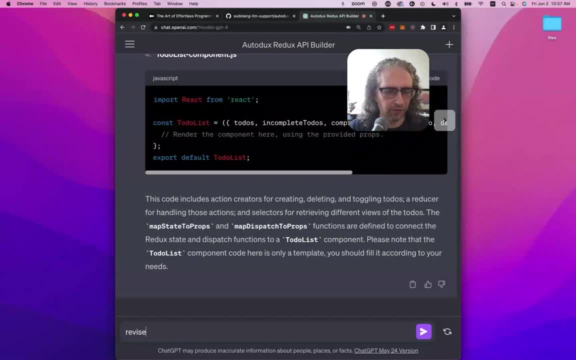 um, revise to-do. in sudo ling we're going to say: add a goal, feature, combine um. so the goal is going to have a to-do list associated with it. so we're going to say: add a to-do list associated with it. so we're going to. 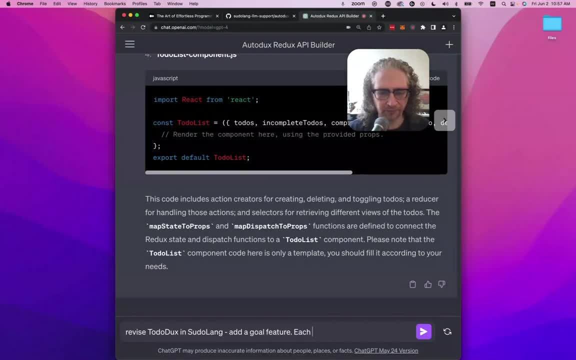 say, add a to-do list associated with it. so, um, each goal will have an associated to-do list and then we can tell it: combine both the goal and the to-do goals and to-do's in the same reducer on the same docs object producing the same reducer. 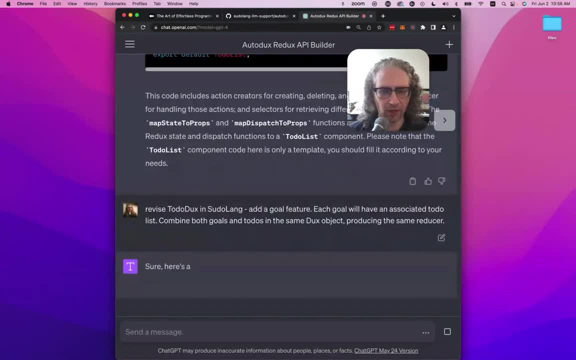 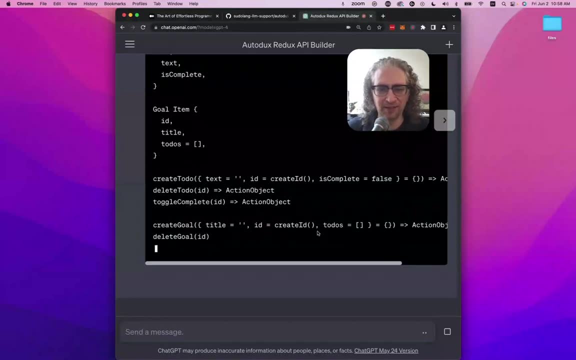 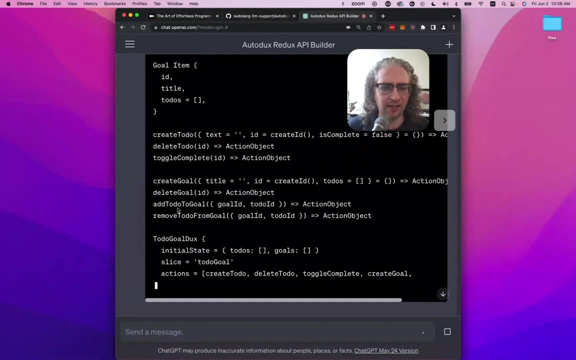 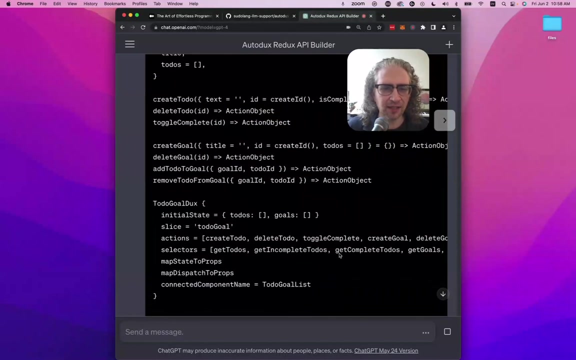 all right. so we tell it that it's going to update our. there we go. so here it's actually producing the sudo link that defines what we're doing. so it's going to have create goal, delete goal. add to-do to goal right. remove to-do from goal. that's nice. um, it looks like. did it get toggle? 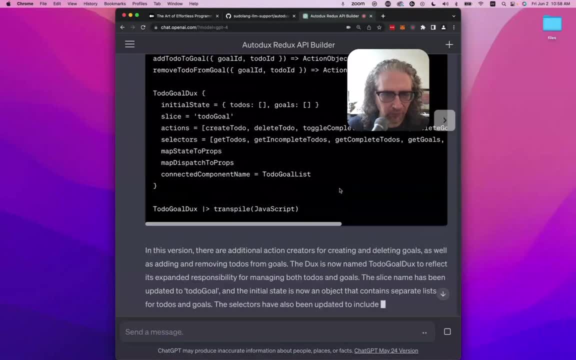 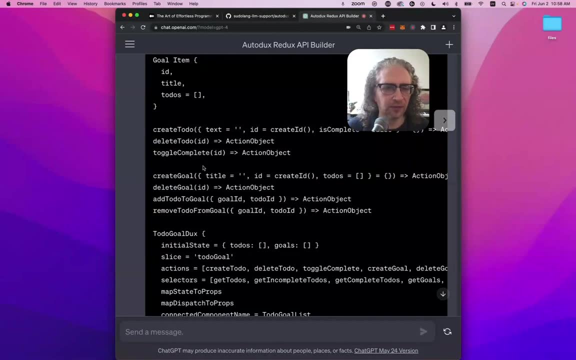 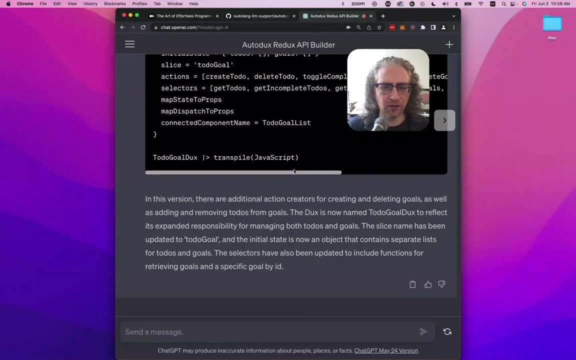 is there a way to toggle: um create, delete. toggle create, delete. add to-do to goal. remove to-do from goal. um, yeah, toggle complete is there? so we're good. so now we should just be able to run transpile and get this new feature completely built out for us. 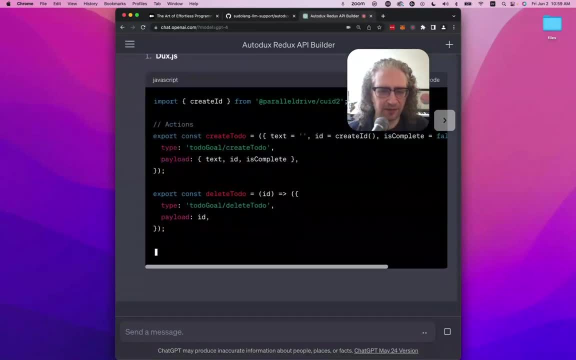 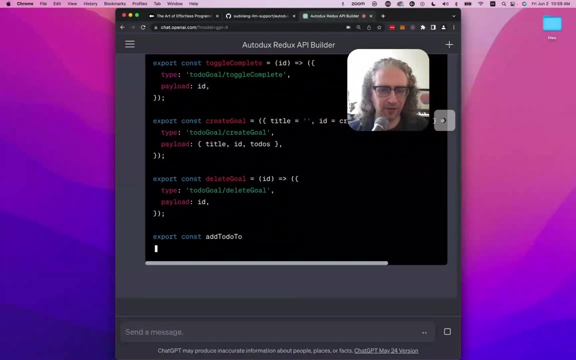 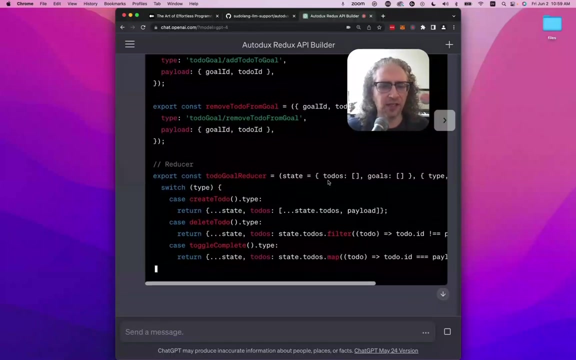 looking good. got our create to do. delete toggle. complete. you create goals, we can delete goals. add a to-do to a goal. remove one from a goal. good, so it looks like our state has to-do's and goals and then the to-do is going to be associated with. 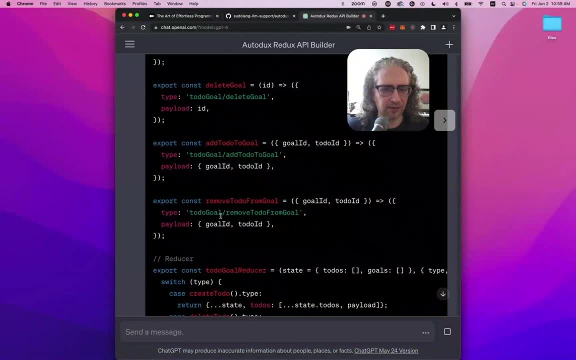 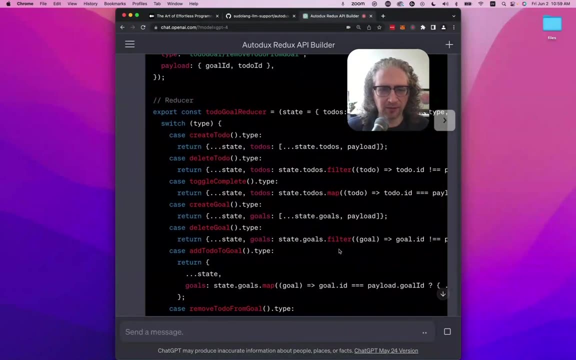 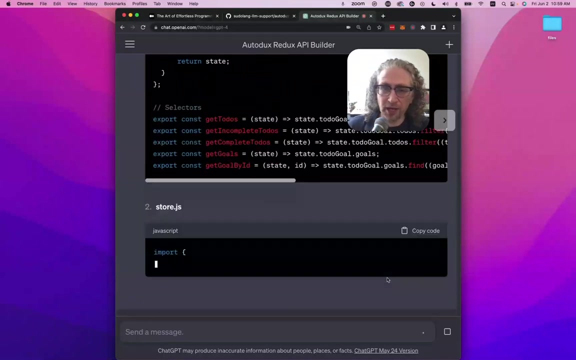 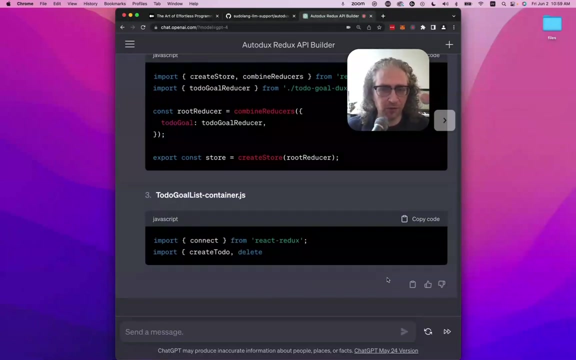 a goal by a goal id. it looks like so? um, yeah, you can see that here. so there we go. all the logic is implemented in just a few seconds. um, we can also ask for a full suite of unit tests. um, like i said, i have another program that. um, that will do. 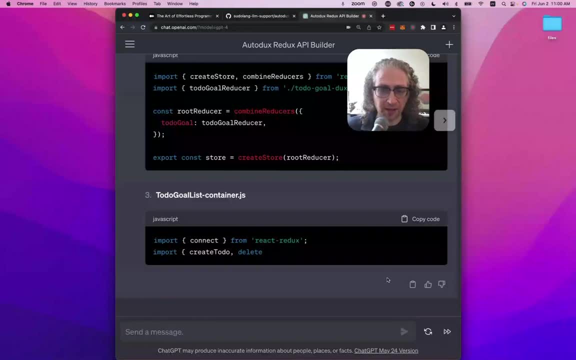 the react components for you, complete with your styles and everything. in fact, that program created the best chat interface i've ever seen. uh, it's very cool. uh, complete with really cool animations. uh, very nice. um, so it can really produce an entire application. uh, in days that. 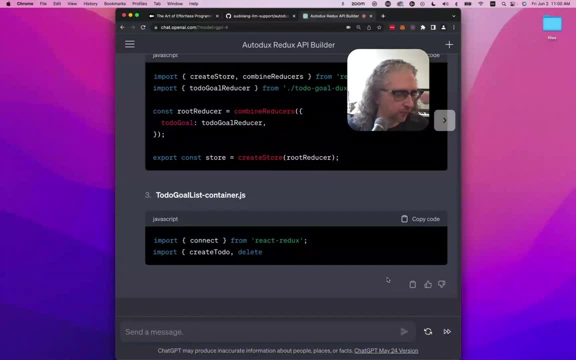 would have taken weeks before and um on the um, even before you get to the coding stage. one of the most important things is to figure out what you're building. i have another program that does that. it just does that, and then you can do that, and then you can do that, and then you can do that.